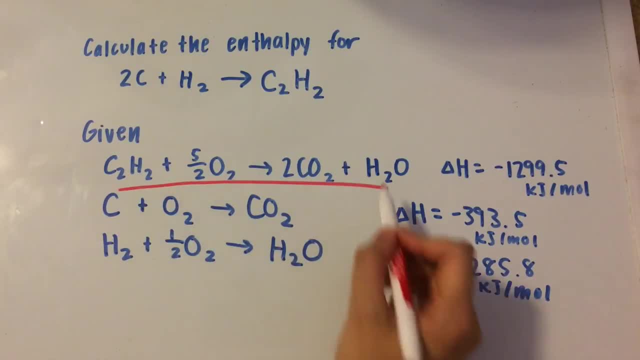 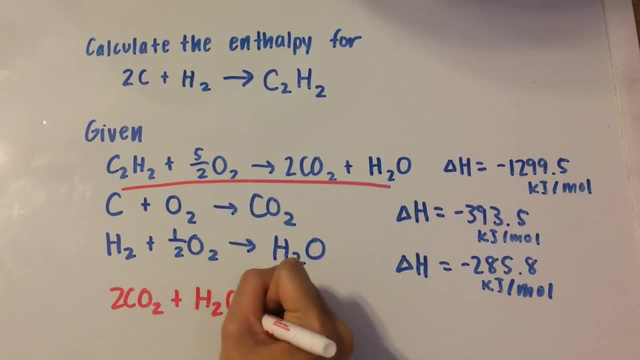 So let's just reverse this whole first equation and that will give us 2CO2 plus H2O yields C2H2 plus 5 halves of O2.. And as you can see, I wrote the delta H's on the side. 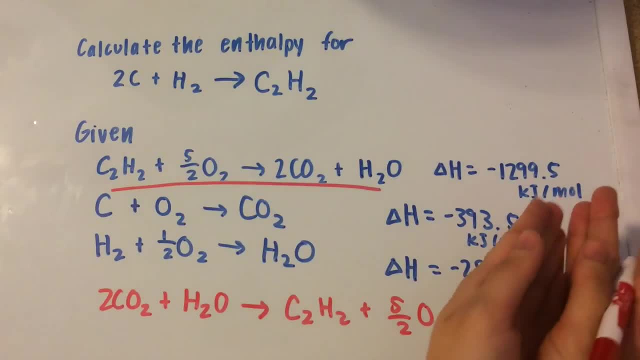 And when we reverse the equation, we need to do the same thing to the delta H or the enthalpy of the reaction. So instead of a negative- 1299.5 kilojoules per mole enthalpy change, we're going to have a positive enthalpy change. 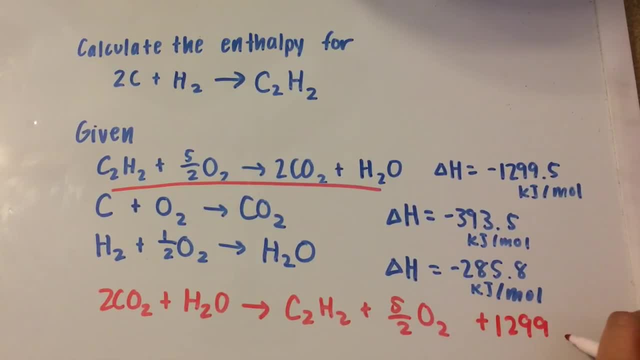 So this is going to be positive: 1299.5 kilojoules per mole of reaction, And a mole of reaction is just this whole equation, right here. Now let's go on to the next one. I see that the carbon is in the same place on the left side of the equation, but we need two moles of the carbon. 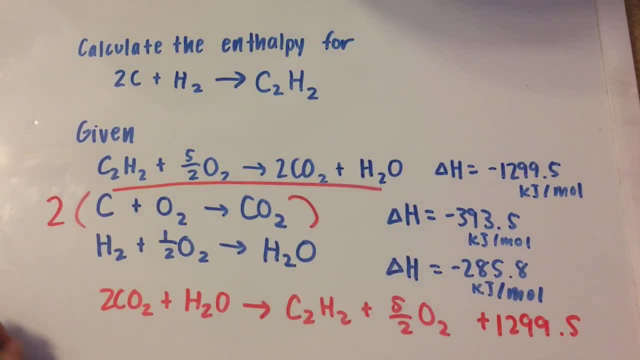 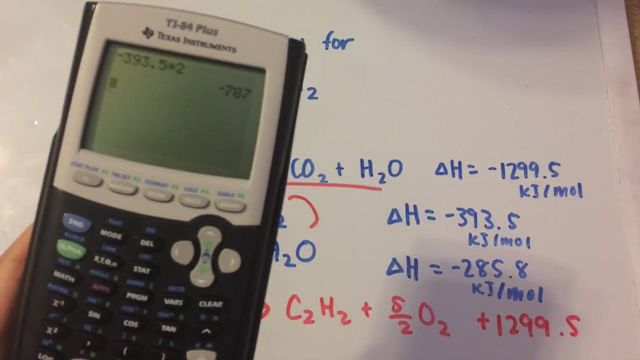 So we have to multiply this whole equation by 2.. And what we do over here is going to be the same thing for the enthalpies. So instead of negative 393.5, we're going to multiply that by 2. Which gives us negative 787 kilojoules per mole of reaction. 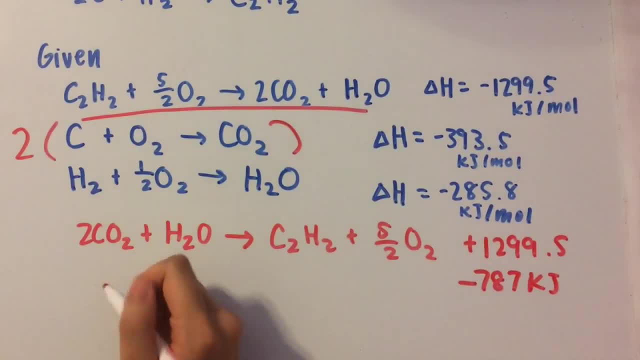 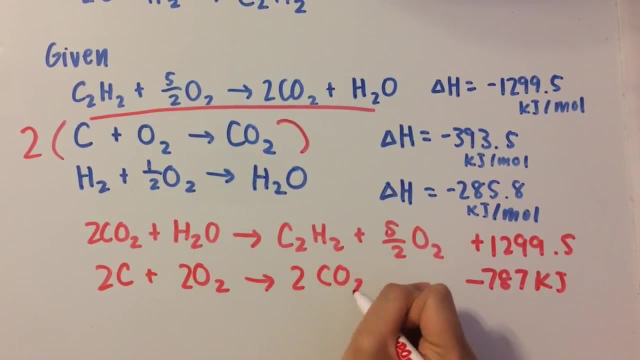 Kilojoules per mole of reaction And we now have 2C plus 202 yields 2 moles of CO2.. Okay, so the last one. I see that we have H2.. It's on the left side of the equation. 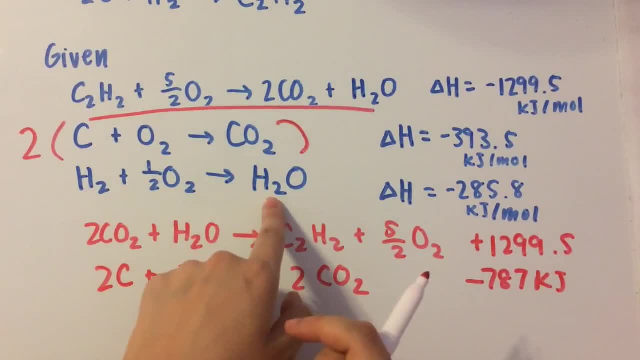 Like we need to multiply that by 2. And we need it to be over here. We could just ignore these and ignore. So it looks like we could just leave this third equation by itself, And I also said that we could ignore these because they're not even in the equation here. 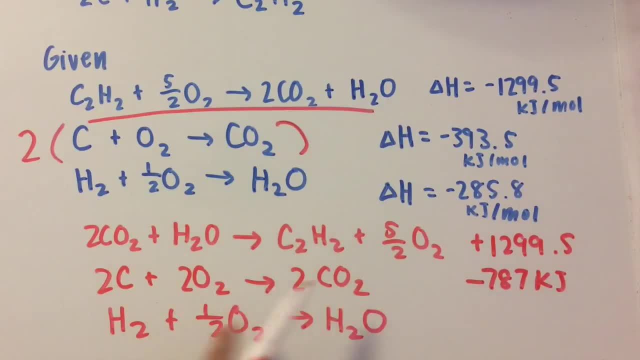 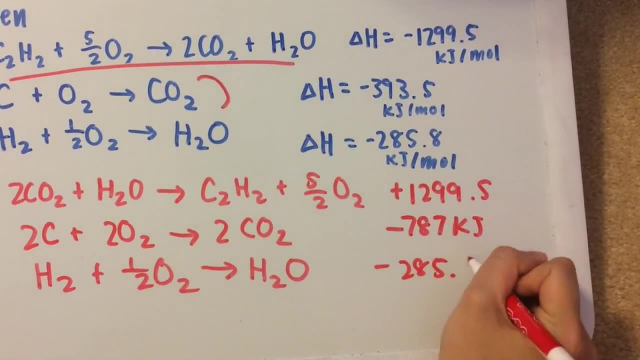 So that's going to tell us that they're probably going to cancel out once we add up these three. So let's see how that works. I forgot to write the enthalpy for this last equation, So let me just write that down.